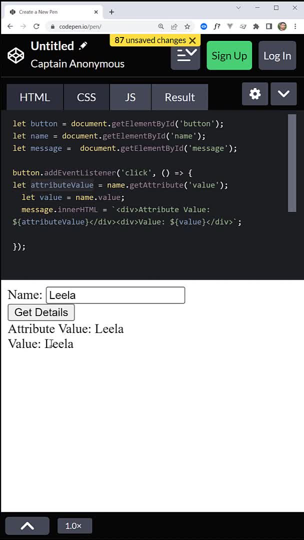 and the value grasping is the same. so the attribute value is giving same, value is giving same. now i will try to update it to leela webday or something like this. now, if i click on this, get details, see that name dot value is giving you the updated, updated value, whereas attribute value is. 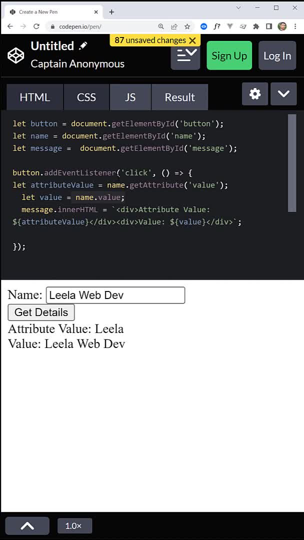 is having only the initial value. so the difference between these two is main: dot get attribute of value, even if you change the input box. also, it will give you the initial default value, what you have added in the html, whereas the dot value will give you the updated details. thank you. 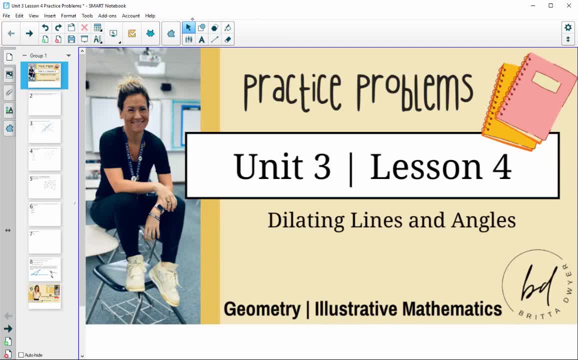 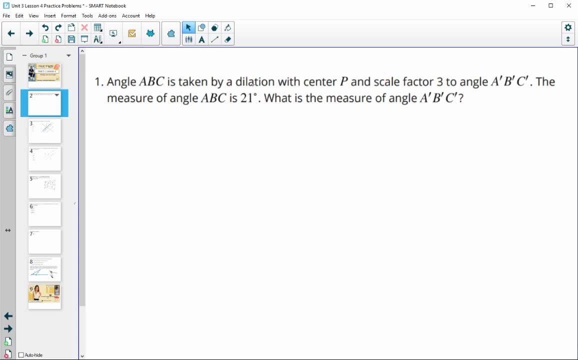 In this video we're going to look at the Unit 3, Lesson 4 practice problems. Number one tells us that we have an angle, ABC, that's being taken by a dilation. They give us the center and the scale factor and it's being taken to A'B'C' The measure of that angle is 21. 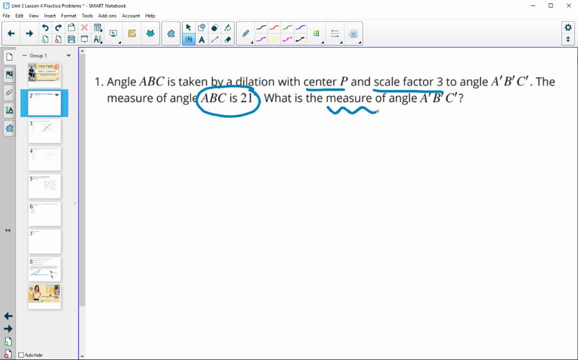 degrees. and then they want us to determine the measure of the dilated angle A'B'C' And when you have a dilation angle, measures don't change. So ABC is going to be the same as A'B'C' So this one's going to be 21 degrees. Number two: select all lines that could be the. 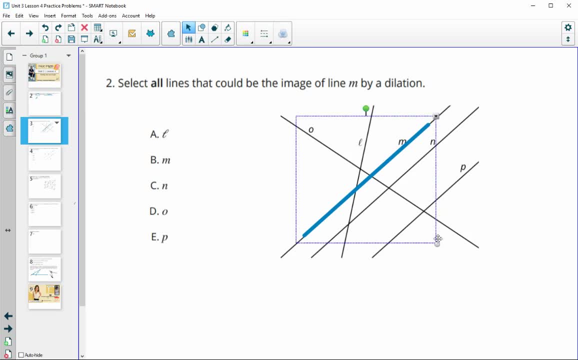 image of line M by dilation. So remember that lines, when they're dilated, can be taken to parallel lines. So if we kind of look at this, here's the dilations of line M, And so we can kind of see that if M were dilated by a scale factor of one, it would be itself. 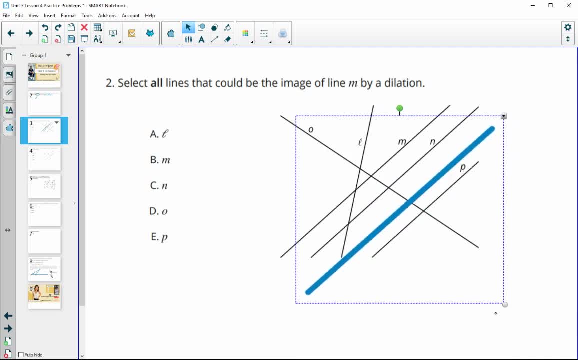 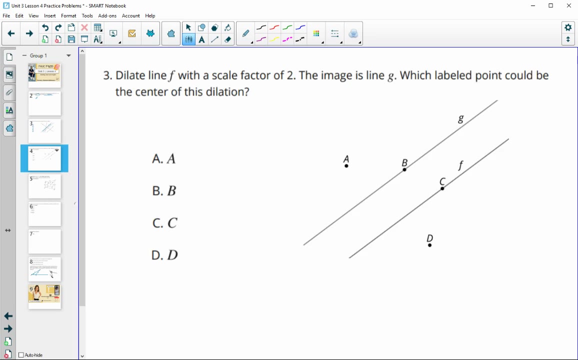 It could go to N, It could also go to P. So those are the three. Could not go to O or L because that would have a rotation with it. So M, N and P. Number three then tells us to, if we dilate line F with a scale factor of two, its 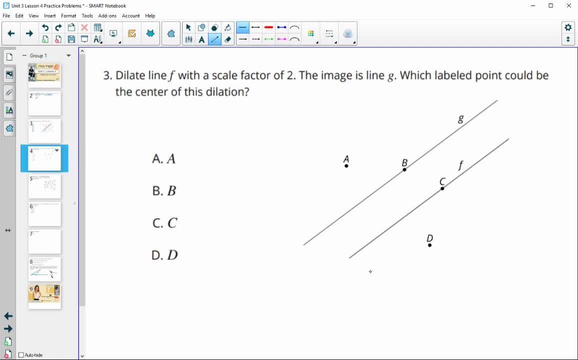 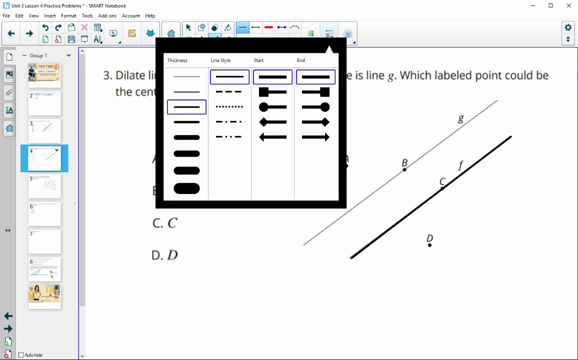 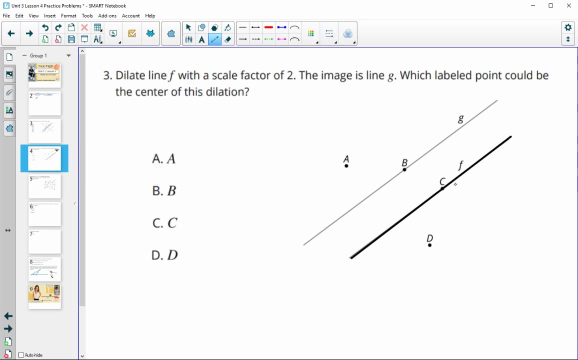 image is G, So F is our original line. so this is our original line and this is being dilated to G. What point could be the center of dilation if we're taking from F to G? So then it's going further away.